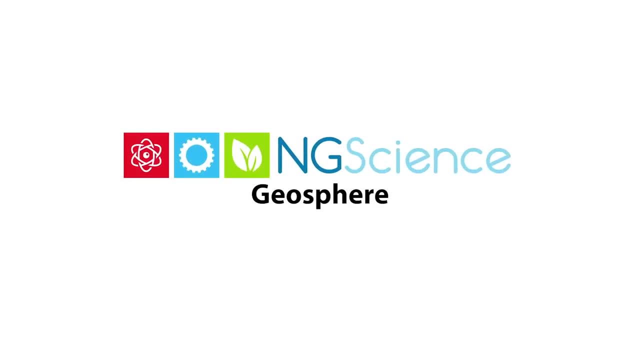 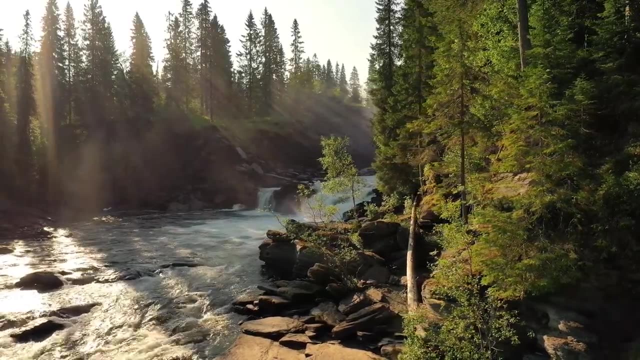 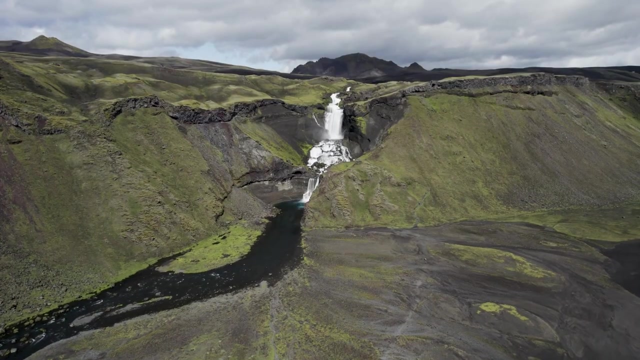 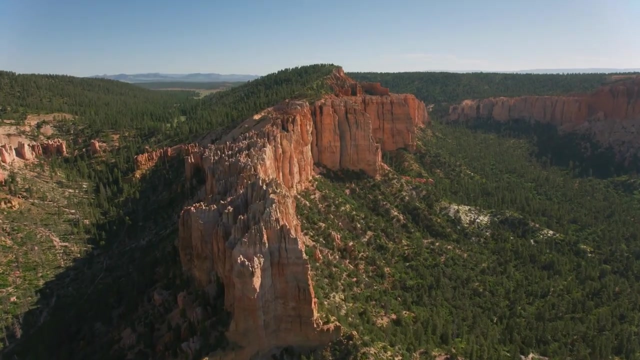 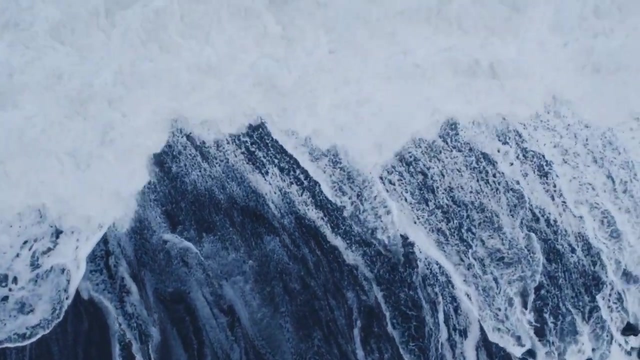 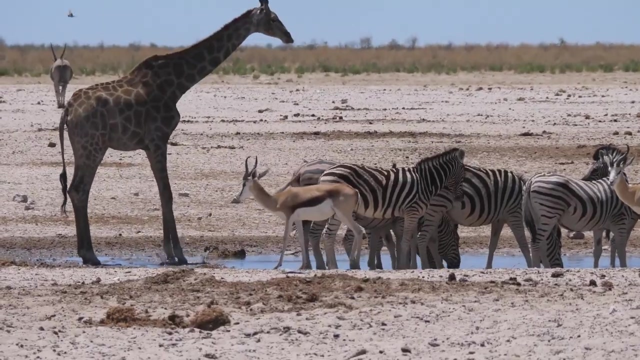 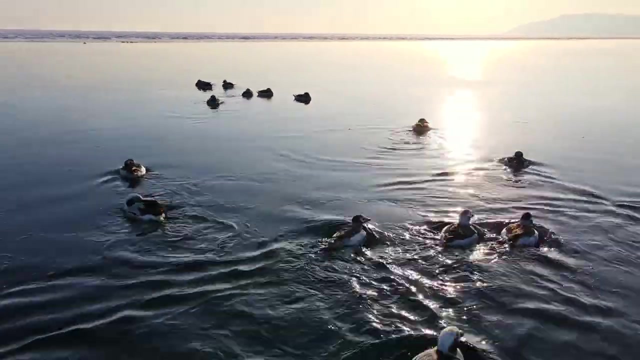 Earth is a complex system composed of four main components or spheres: The geosphere, solid earth, hydrosphere, water, atmosphere, air and biosphere- life. Each of these spheres interact with each other, influencing Earth's climate, landforms. 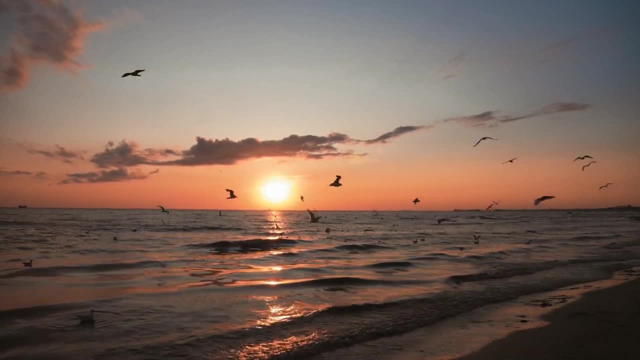 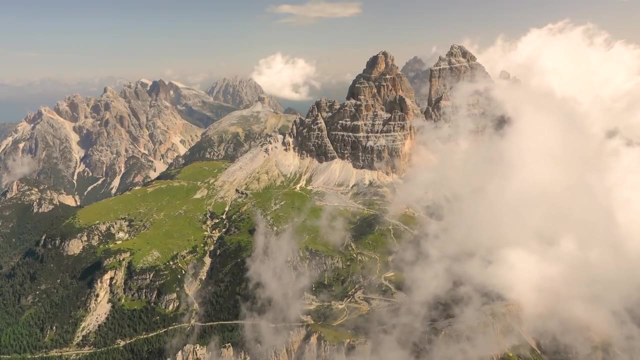 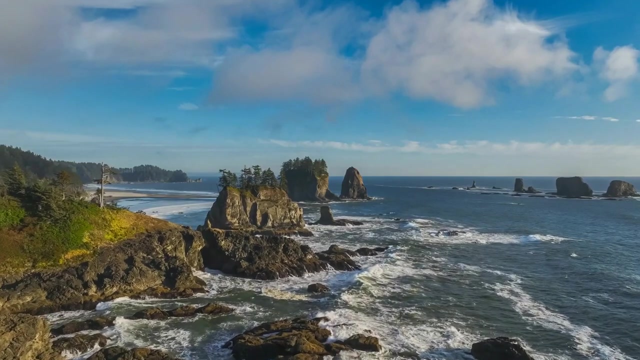 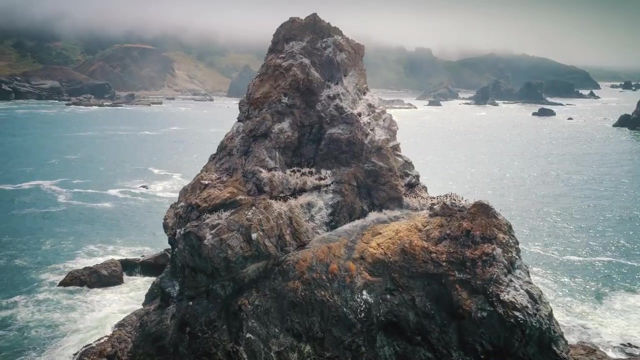 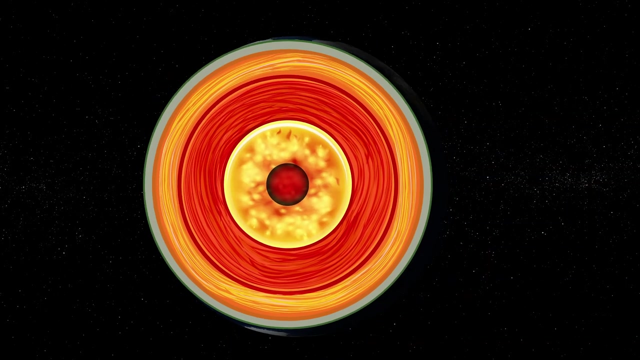 and lifeforms. The geosphere is all the solid matter that makes up our planet. extending from the Earth's surface down to its core. It comprises rocks, mountains, beaches and all the other physical features, excluding water and living things. This includes not just the Earth's surface, but also the layers beneath it, the crust. 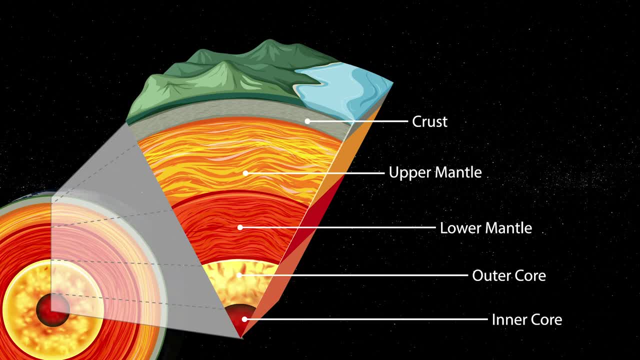 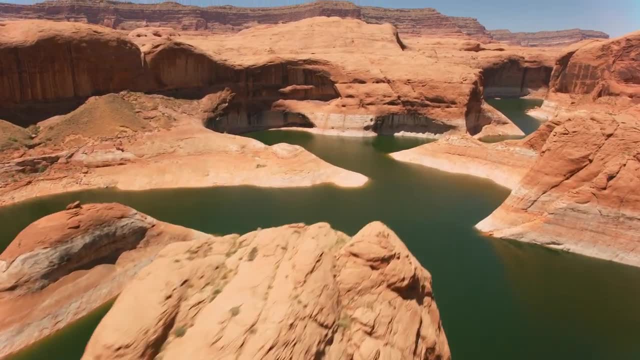 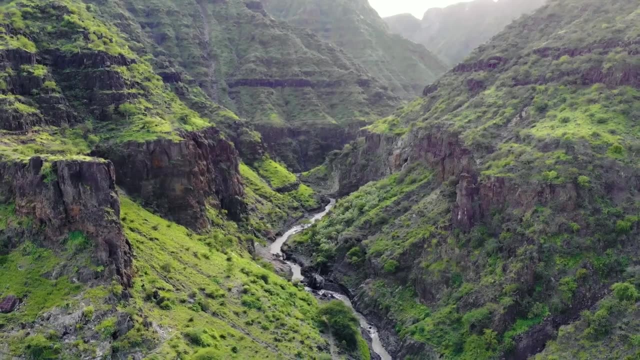 mantle and core. The geosphere interacts with the other spheres in many ways. For example, it interacts with the hydrosphere, as rivers shape valleys and create sediment, or when heat from the Earth's core warms the atmosphere. Otherwise, these drawings interact with our generated energy and when direct drove by 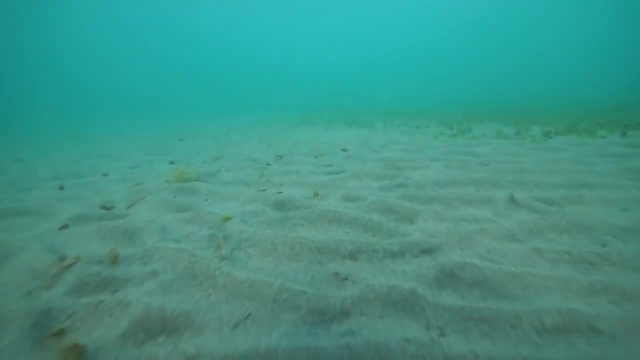 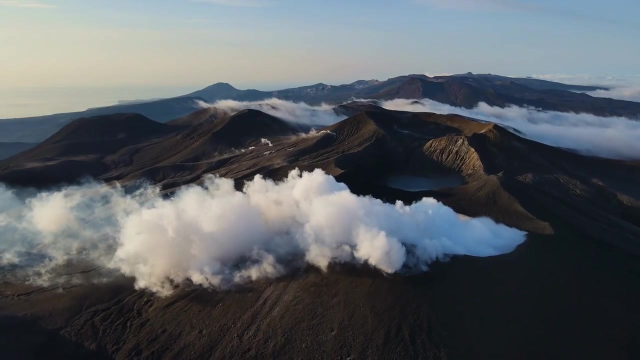 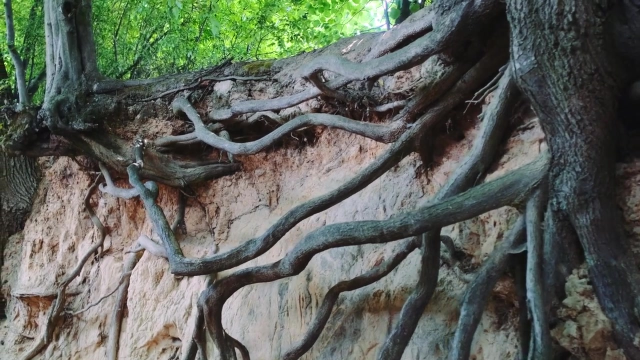 the heat of the movement of the spirals forms the bottom of oceans. The interactions with the atmosphere occur when volcanic eruptions from the geosphere release gases into the atmosphere, influencing climate With the biosphere. the interaction happens when plants break down rocks into soil or 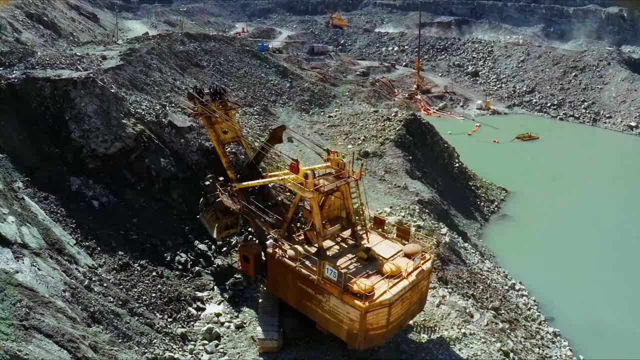 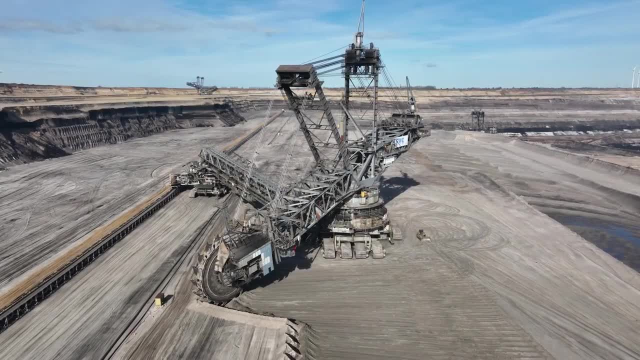 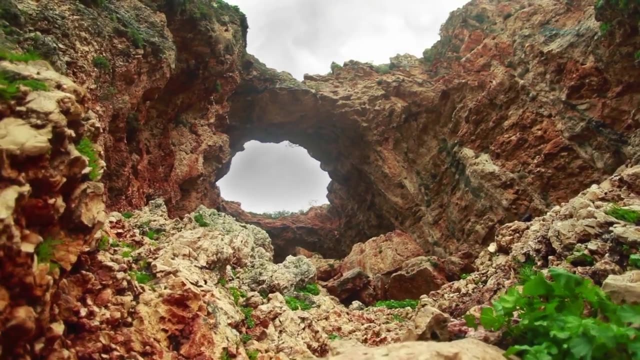 when humans excavate the geosphere for resources such as minerals and metals. These activities not only affect the geosphere, but can also impact the other spheres. The Earth's geosphere, while primarily composed of the solid parts of the Earth, is interconnected.